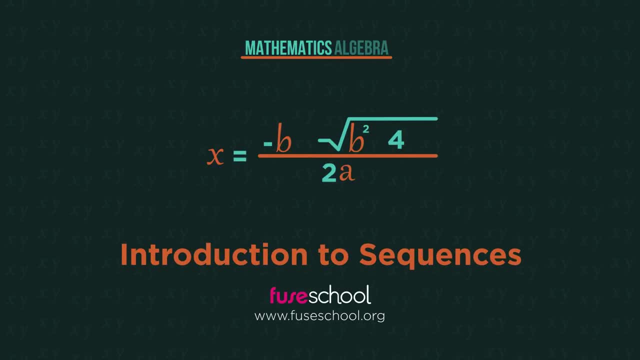 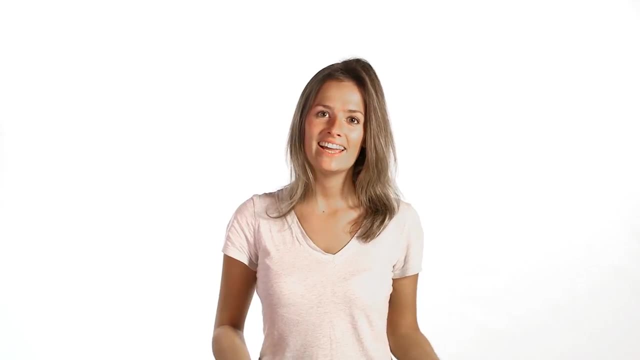 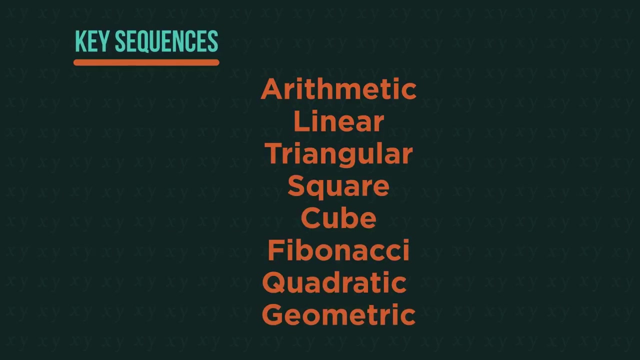 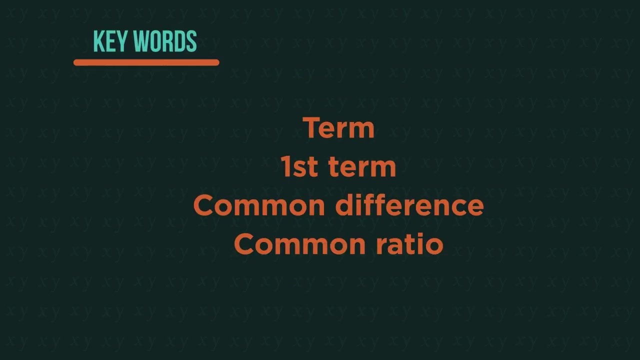 In this video we're going to discover some key sequence terminology and how to recognise and generate some important sequences. We will come across all of these key sequences and these keywords. Each number in the sequence is called a term. This is the first term, second term, and so on. This just tells us that the 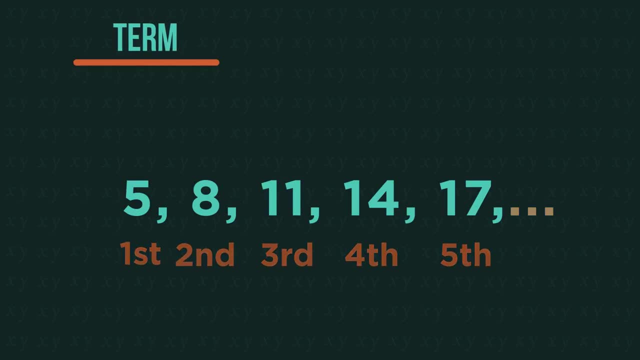 sequence carries on forever. This sequence is very easy to carry on. We can easily spot it's going up by three each time Because it's plus three every time. we say it has a common difference of three Sequences that have a common difference- so the same difference every time- are called: 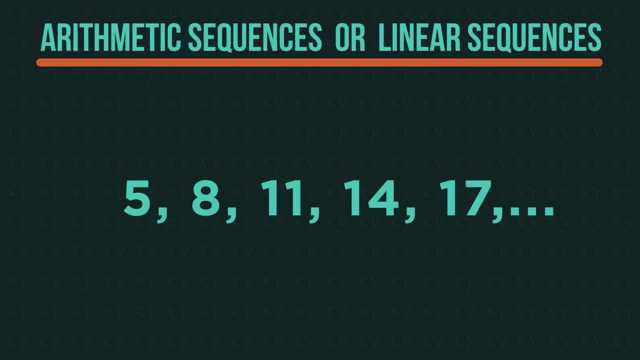 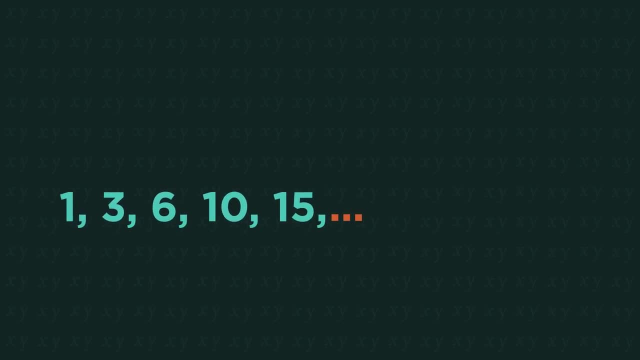 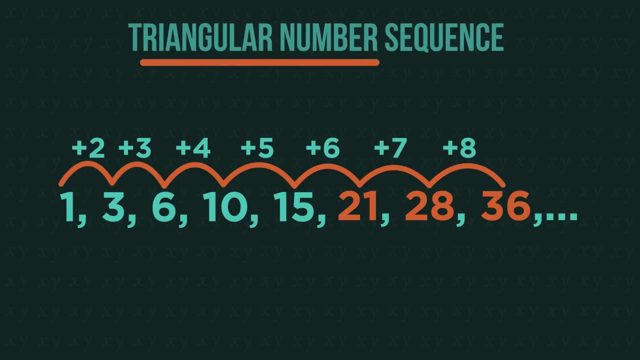 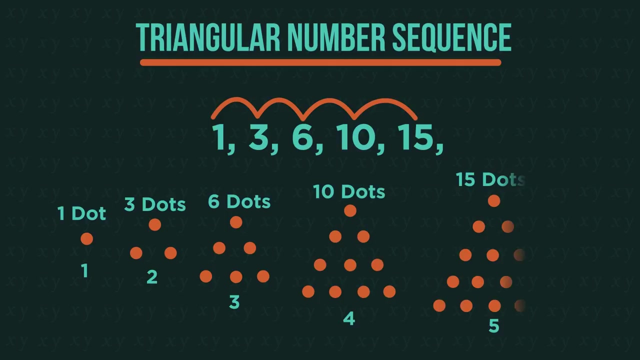 arithmetic Sequences or linear sequences. Can you find the next three terms of this sequence? Did you get 21,, 28 and 36?? These are the triangular numbers or the triangular number sequence. The sequence comes from the pattern of dots needed to 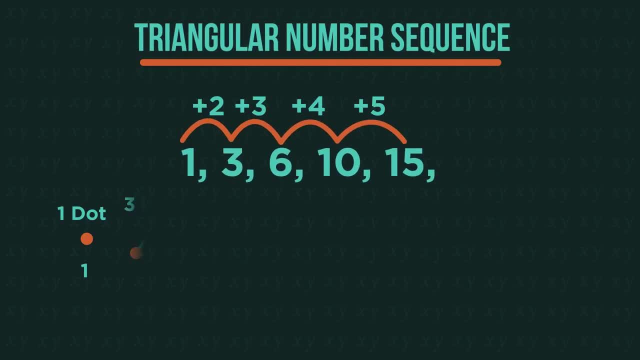 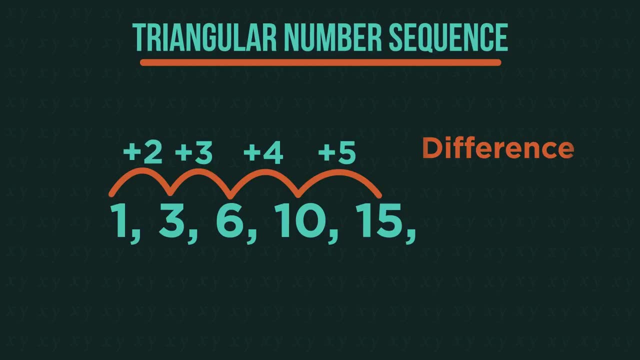 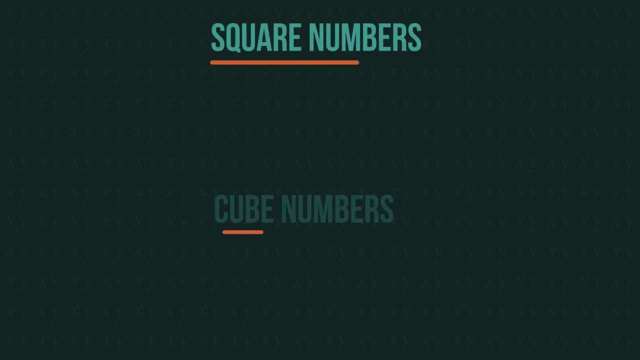 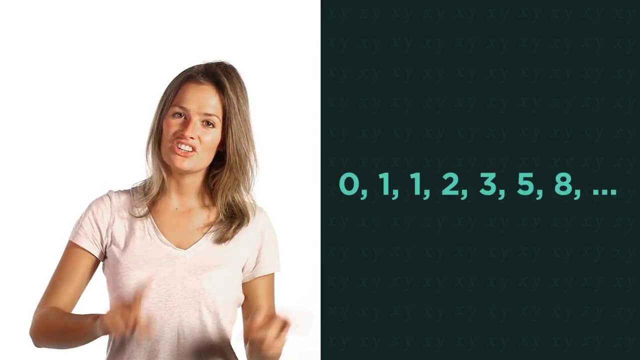 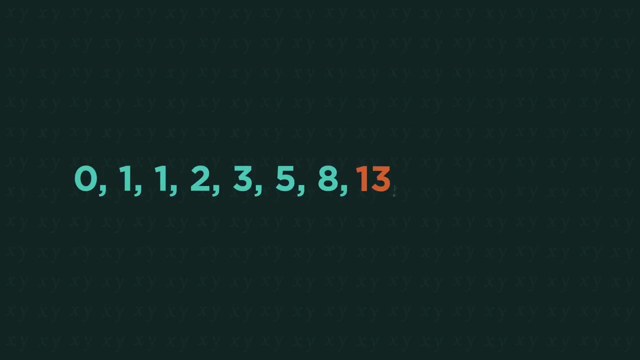 make a triangle. They don't have a common difference. The difference changes each time. You add two, then you add three, then four, then five. Square numbers and cube numbers are also special sequences. But what about this special sequence? Can you find the next three terms? Did you get 13,, 21 and 34?? 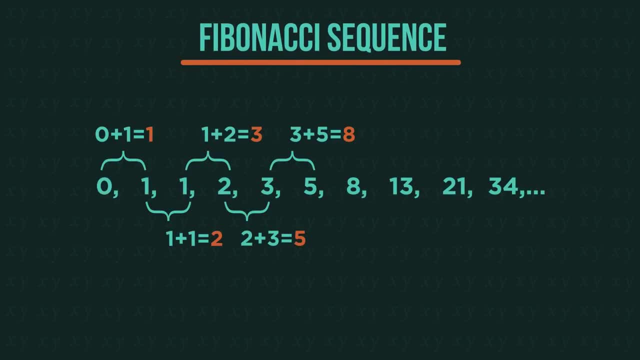 This is called the Fibonacci sequence. You just add up the two numbers before to get the next term. There's a lot you can discover about Fibonacci 515 00 kijken, Such as: if you make squares of Fibonacci sizes, You get a spiral. 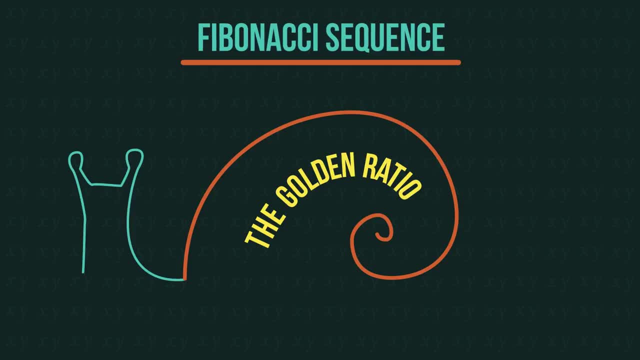 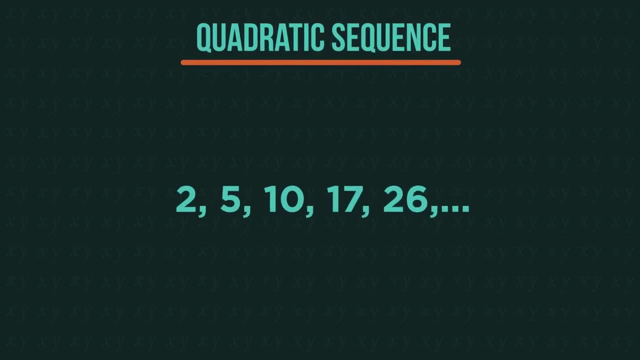 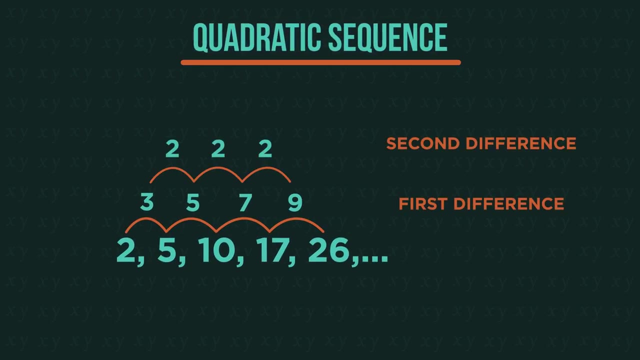 It's also linked to the golden ratio and is seen throughout nature. 6: foettig: This is a quadratic sequence. If we look at the difference, It isn't the same same, But if we look at the second difference it is the same, which means it's a quadratic.